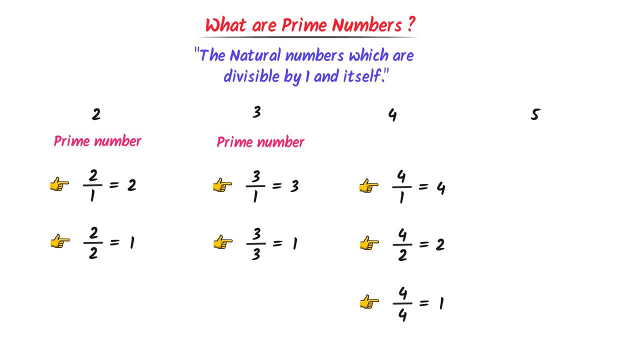 is also it. 4 by 4, we get 1.. Hence we can divide 4 by 1,, 2 and itself It has more than 2 divisor, hence it is not a prime number. Fourthly, we can divide 5 by 1, we get 5. And we can. 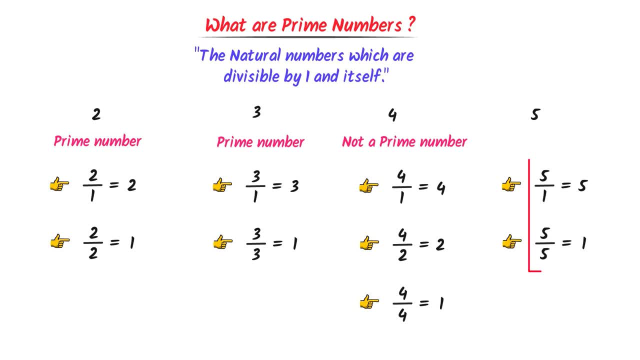 divide 5 by 5, we get 1.. It has only 2 divisor. it is a prime number. Thus, remember that prime numbers are those numbers which are divisible by 1 and itself. Now let me teach you some important questions of prime numbers. Is 1 a prime number? The 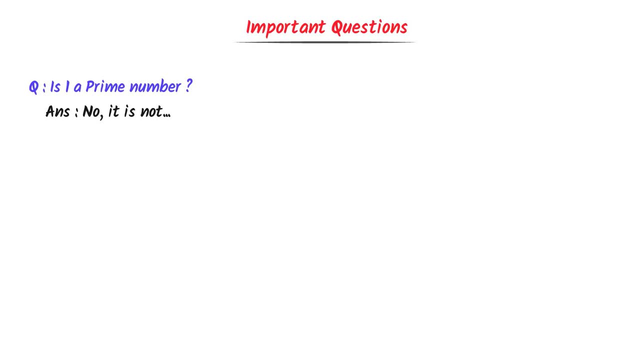 answer is NO. 1 is not a prime number. For example, we can only divide 1 by 1, it has only 1 divisor. We know that every prime number has 2 divisors, hence 1 is not a prime number. 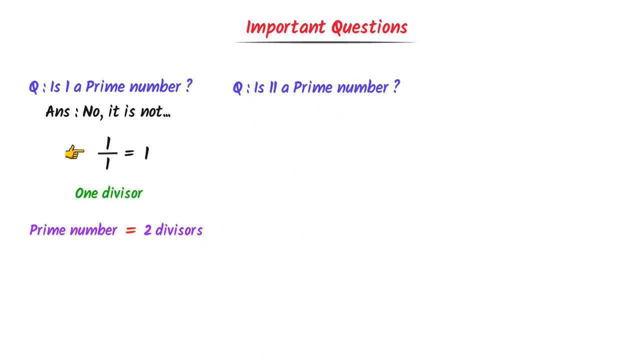 OK, OK. Secondly, is 11 a prime number? The answer is yes, 11 is a prime number. We can divide 11 by 1 and we can divide 11 by 11.. It has two divisors. hence, 11 is a prime number. 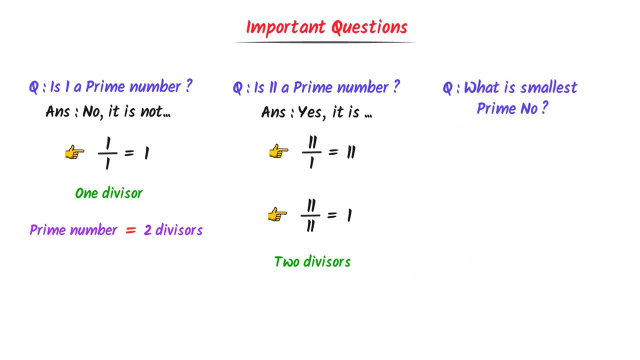 Thirdly, what is the smallest prime number? The answer is 2,. 2 is the smallest prime number. Fourthly, what is the largest 4-digit prime number? The answer is 9,973.. It is the largest 4-digit prime number. 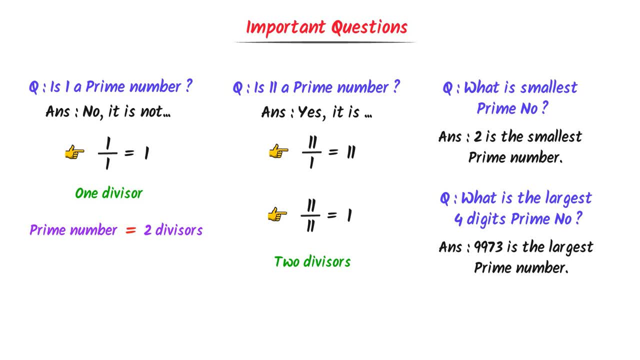 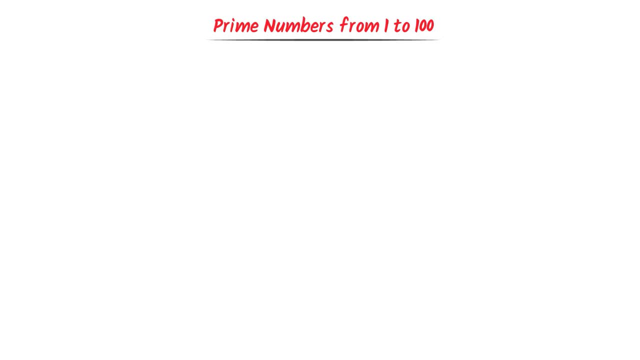 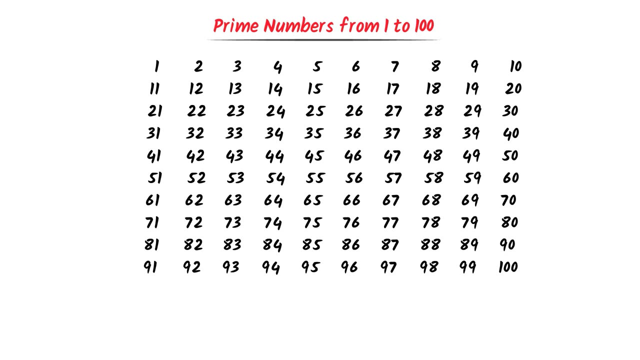 So note it down, all these important questions. Now let me teach you prime numbers from 1 to 100.. I will teach you my personal trick, which you cannot find anywhere. Firstly, I write numbers from 1 to 100.. We already know that 1 is not a prime number. 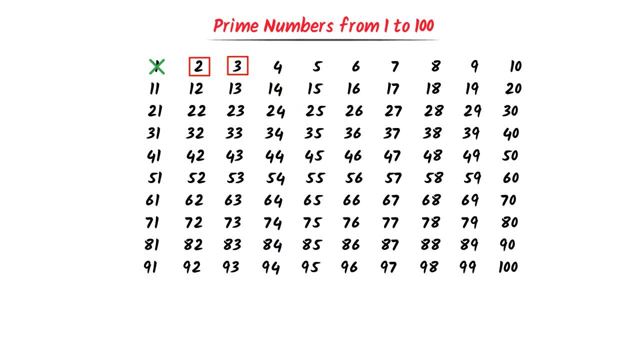 Secondly, 2 is a prime number, 3 is a prime number, 5 is a prime number, 7 is a prime number. On the other hand, 4, 6,, 8,, 9,, 10 are not prime numbers. 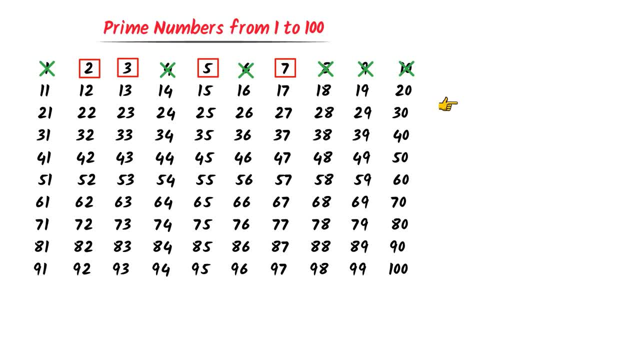 Now I just follow 4 steps in order to find all the prime numbers. The first step is to cut the numbers. The first step is to cut the numbers. The first step is to cut the numbers. The second step is to cut the multiples of 3.. 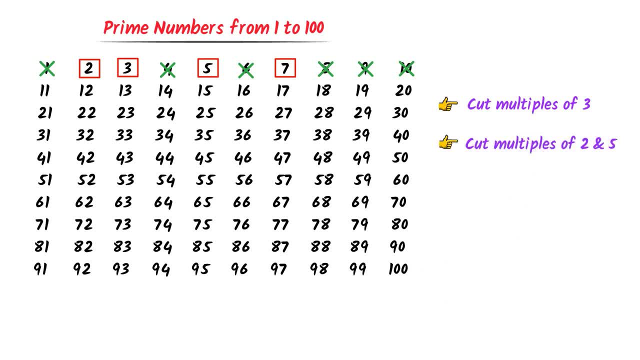 The second step is to cut the multiples of 2 and 5.. The third step is to cut 49 and 91.. The fourth step is to cut the multiples of 11 diagonally. Now, according to the first step, we have to cut the multiples of 3.. 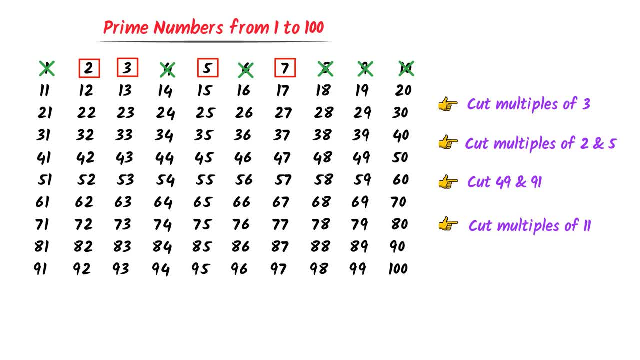 I start from 3 and count 3 times: 1,, 2, 3.. I cut 8.. Then 1, 2,, 3.. I cut 8.. I will use this pattern to cut every third number. 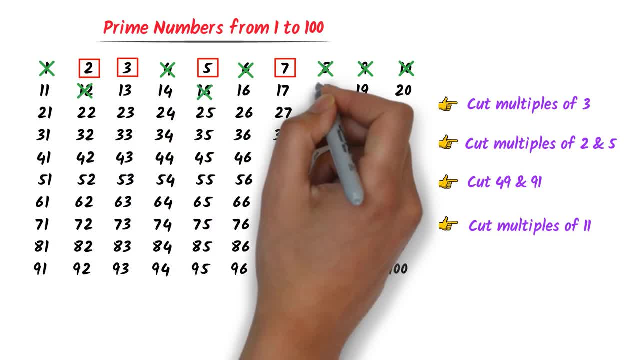 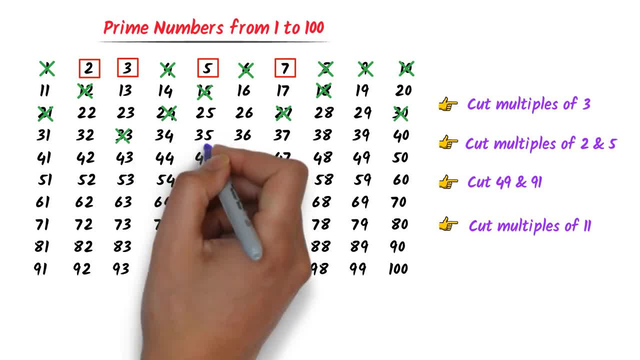 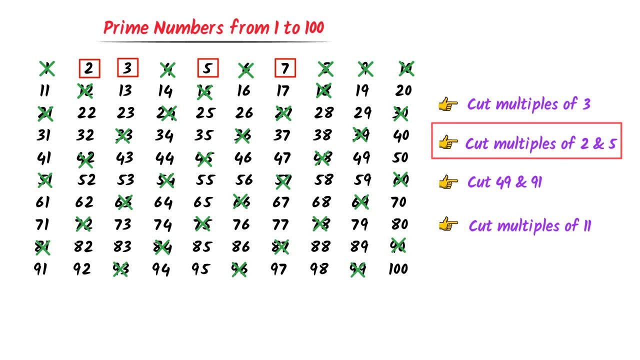 1, 2, 3.. 1, 2, 3.. 1, 2, 3.. And so on. According to the second step, I have to cut the multiples of 2 and 5.. Now this column is a prime number. 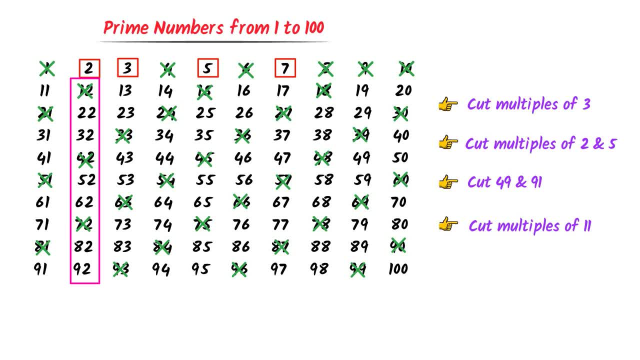 The second step is to cut the multiples of 2 and 5.. Now, this column is a prime number. The second step is to cut the multiples of 2 and 5. This column is a prime number. This column is a prime number. 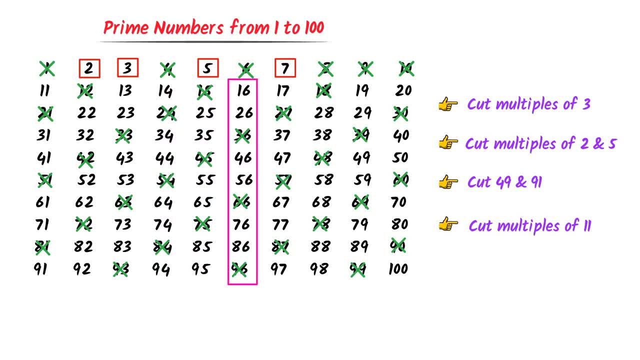 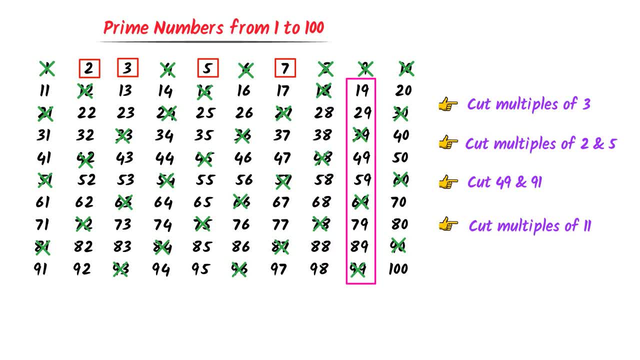 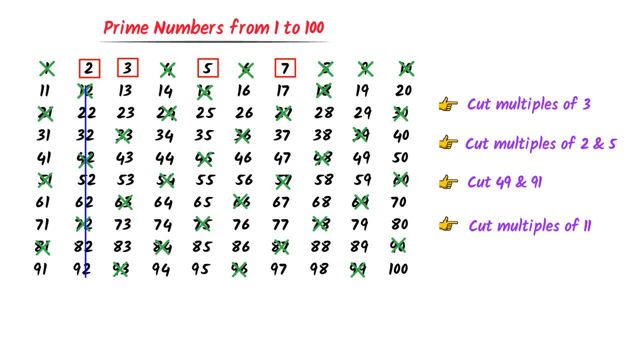 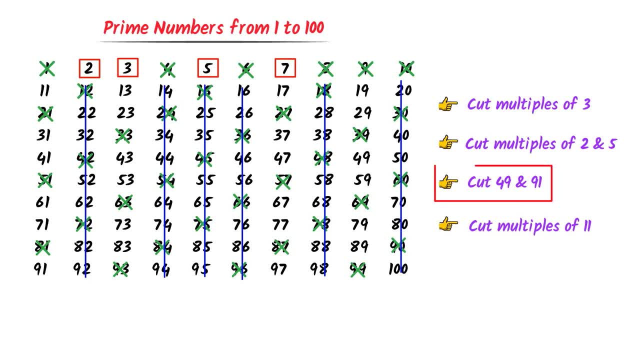 I also cut this column. According to the 3rd step, cut 49 and 91.. Lastly, according to the 4th step, cut the multiples of 11 diagonally like 22,, 33,, 44,, 55,, 66,, 77,, 88,, 99. 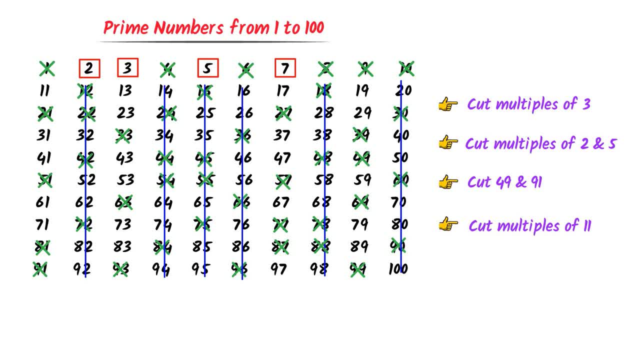 So these all remaining numbers are prime numbers: 2,, 3,, 5,, 7,, 11,, 13,, 17,, 19,, 23,, 29,, 31,, 37,, 41,, 43,, 47,, 53,, 59,, 61,, 67,, 71,, 73,, 79,, 83,. 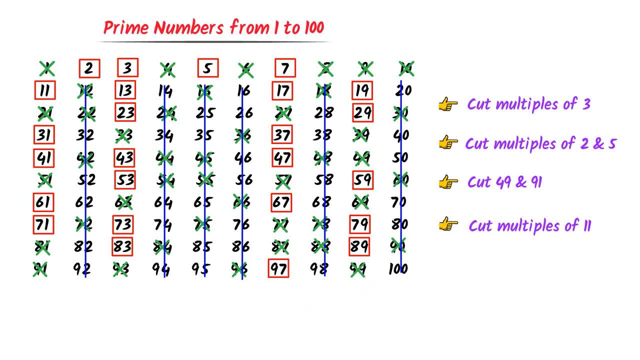 89, 97.. So everything is just prime numbers. Now the prime numbers from 1 to 10 are 2,, 3,, 5, and 7.. First早就要做 saham. Now the prime numbers from 1 to 10 are 2,, 3,, 5, and 7.. 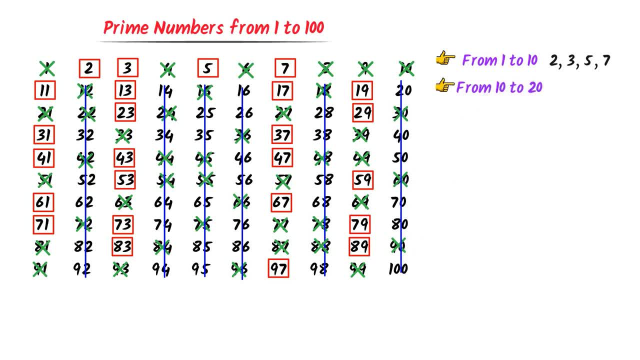 The prime numbers from 10 to 20 are 11,, 13,, 17, and 19.. The prime numbers from 20 to 30 are 23 and 29.. The prime numbers from 30 to 40 are 31 and 37.. 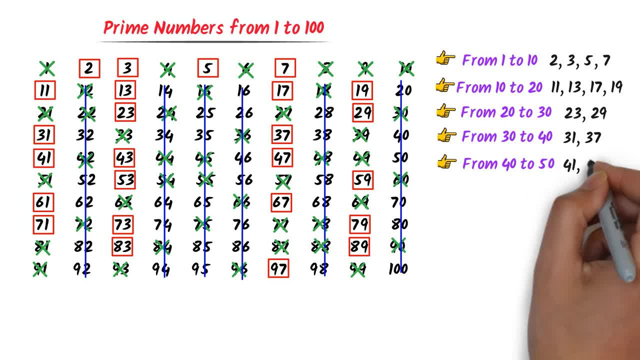 The prime numbers from 40 to 50 are 41 and 48.. 캐�cards being apart from one another: pi 43, and 47.. The prime numbers from 50 to 60 are 53 and 59.. The prime numbers from 60 to 70 are: 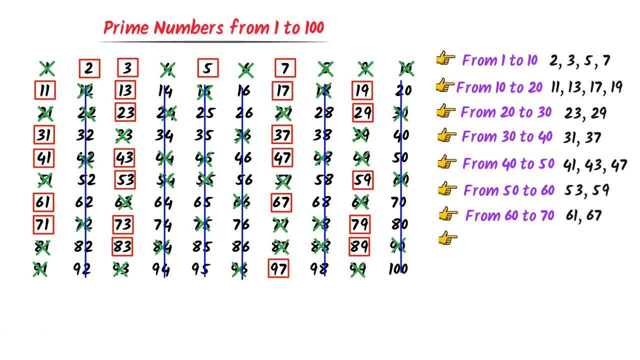 61 and 67.. The prime numbers from 70 to 80 are 71,, 73, and 79.. The prime numbers from 80 to 90 are 83 and 89.. The prime numbers from 90 to 100 are 97.. Hence, these are the prime numbers from 1 to. 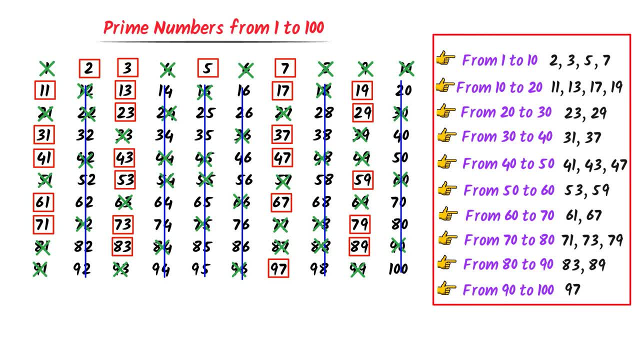 100.. Now if I count these prime numbers from 1 to 100, they are total 25 numbers. Usually an exam, it is asked as: how many prime numbers are there between 1 and 100?? Well, the answer is: